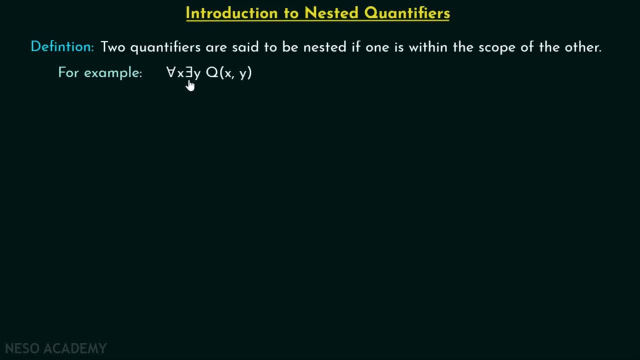 One is for all and the other one is there exist. There exist is coming within the scope of for all. So we can say these two are nested quantifiers. Here you can see that there exist is coming after for all. We can say that there exist is within the scope of for all. 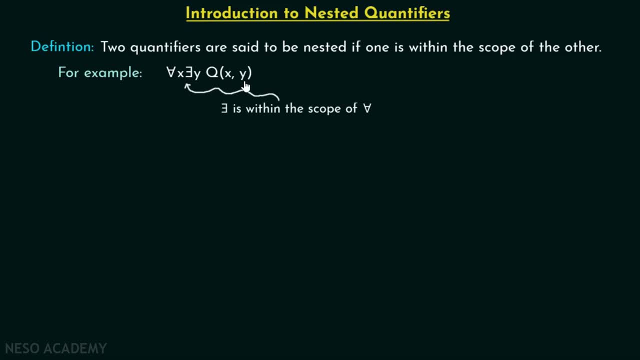 After this we have a propositional function that is qxy. That's not a problem. Please note that anything within the scope of the quantifier can be thought of as a propositional function. We know that there exist y. qxy is coming. 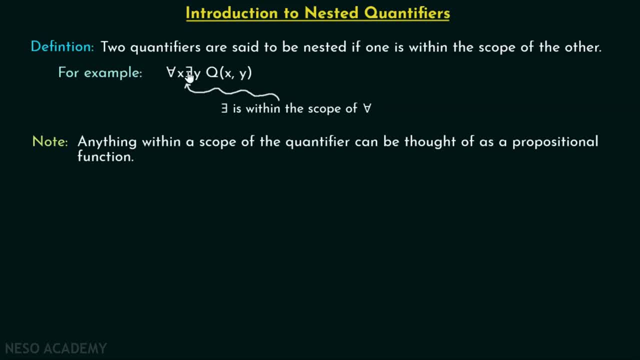 under the scope of this quantifier for all. So we can replace this by some propositional function. That is why I have replaced there exist y, qxy by this propositional function px. This p can be replaced by anything, That's not a problem. 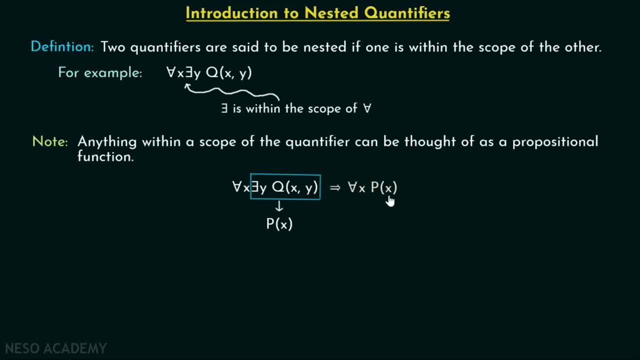 So we can write this as for all x px, Instead of writing for all x: there exist y, qxy. There exist y, qxy. we can also write this as for all x px. Later we can expand px to: there exist y, qx, y. 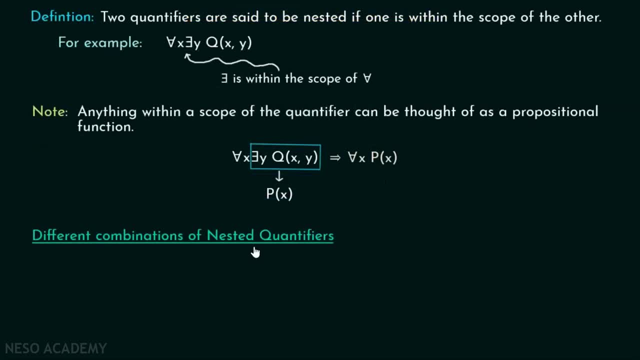 That's not a problem. right Now, let me tell you. there are different combinations of nested quantifiers available. Here you can see I am considering all four combinations. okay, Because we have two quantifiers. we can arrange them accordingly. That is why we can obtain four different combinations. 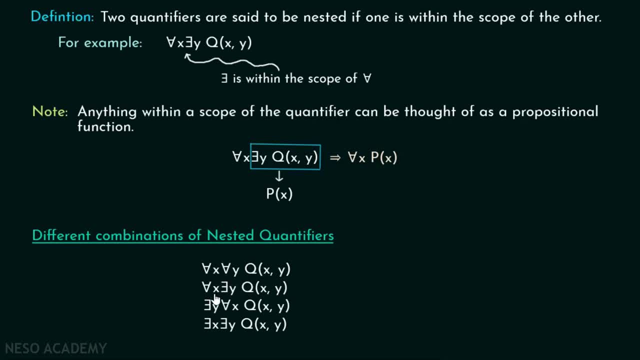 Here. the first one is for all x, for all y, qx, y, For all x. there exist y, qx, y, There exist y. for all x, qx, y, There exist x, there exist y, qx, y. 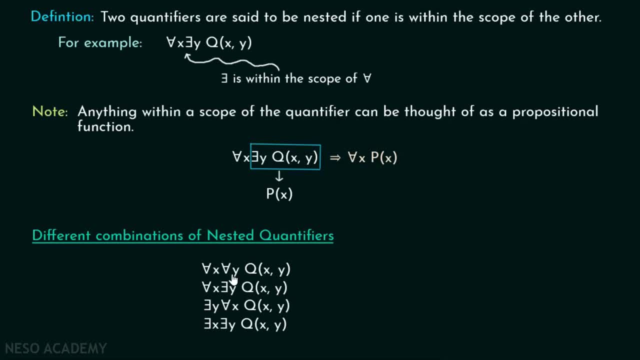 Let me tell you, for the first one and the last one, the order doesn't matter at all. okay, The order of quantifiers for the first as well as last one doesn't matter at all. We can change the order of these quantifiers. 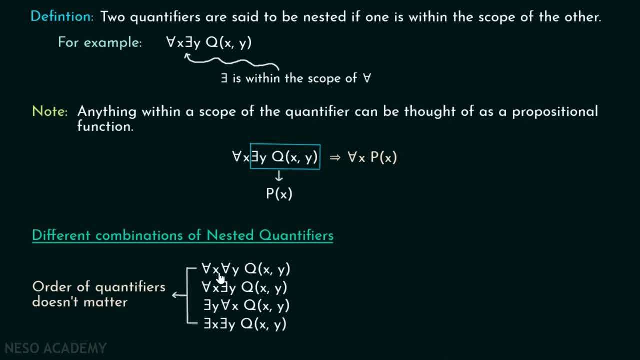 That means we can write for all y for all x in place of for all x for all y. We can also write there exist y, there exist x in place of there exist x, there exist y. That's not a problem. 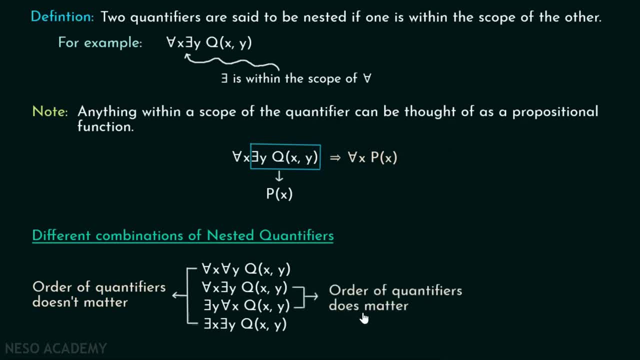 But for the middle two, the order of quantifiers does matter. okay, For all x, there exist y cannot be written as there exist y for all x. We cannot change the order here. okay, Therefore, for all x, there exist y and there exist y for all x are two different things.